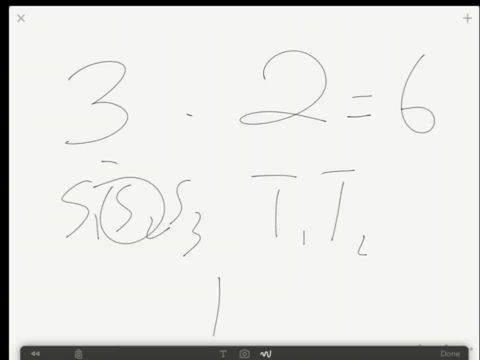 And a trouser. okay, Having done that, now let's be a little bit more formal and define two rules, of two basic rules which are very, very common sense. The first rule is The rule of sum. The rule of sum. 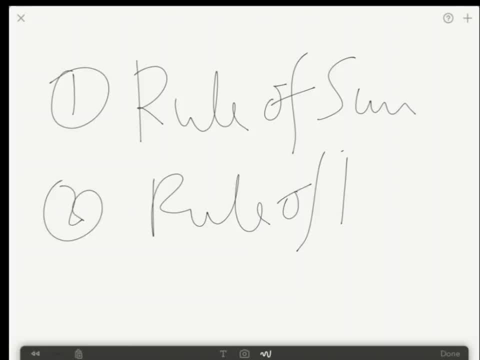 And the second rule is the rule of product, So the rule of sum. The best way to understand this is by an example, If you have to, there are. so imagine there are three airports: Airport A, Airport B and Airport C. 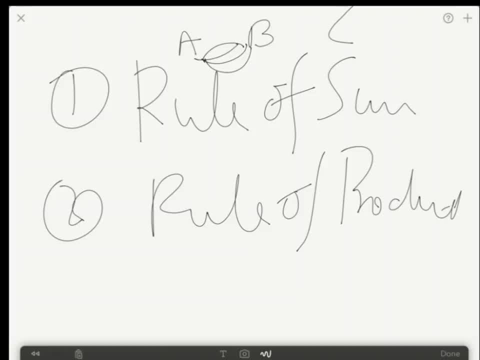 And there are four ways to go from Airport A to Airport B and there are three ways to go from Airport B to Airport C And, if I ask the question, how many ways are there to get out, get out of, Get out of airport? 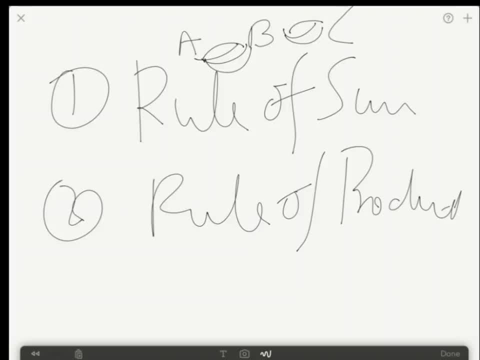 How many ways are there to get out of Airport B? So you would say: okay, there are four ways to get out of Airport B. So there are these four ways and there are three ways to get out of Airport B to C. 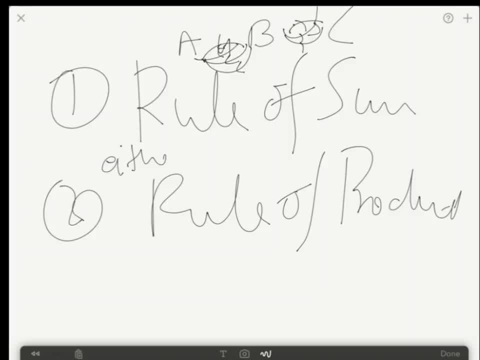 So there are three other ways. So you say: either I take these four routes or you take the other three routes. So in total you have three plus four or four plus three, which is seven. So here this: 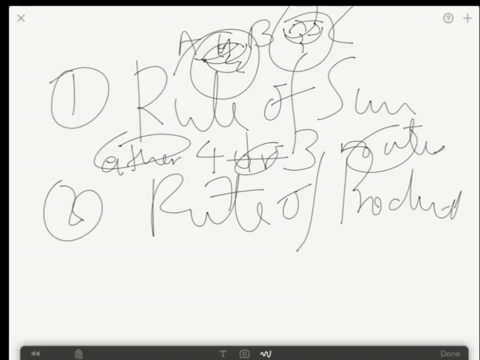 Either or converts into an addition. So in general, if you have A ways to do something and B other ways of doing the other thing, then you have A plus B ways of doing the entire activity. I'm going to say that again. 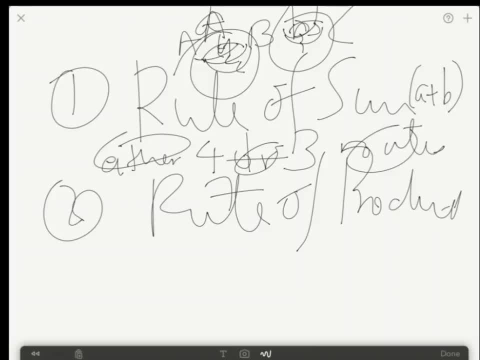 If there are A ways of doing an activity and there are B other ways of doing the same activity, then the activity can be done in A plus B ways. So that is the rule of sum. Now, if I ask, I'm going to ask you the same question, but give it just a slight twist. 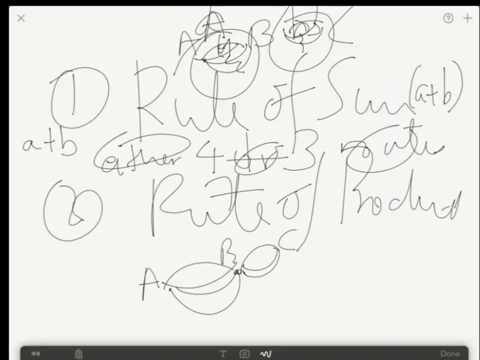 in which I ask: how many ways are there to go from Airport A to Airport C, So from A to C? Then you would say: there are four ways of going from A to B, right? And there are three ways of going from B to C, right? 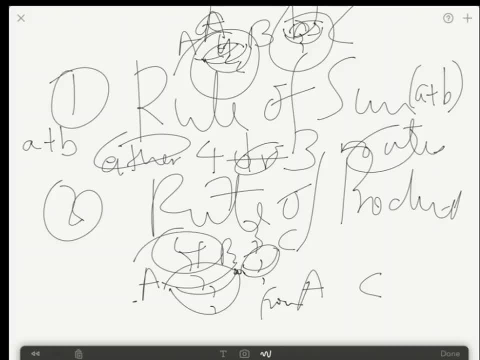 And for each of the ways that you can go from A to B. there are three ways of going from B to C. No matter which way I choose of going from A to B, there are three ways of going from B to C. So these choices, the four choices and these three choices are independent of each other. 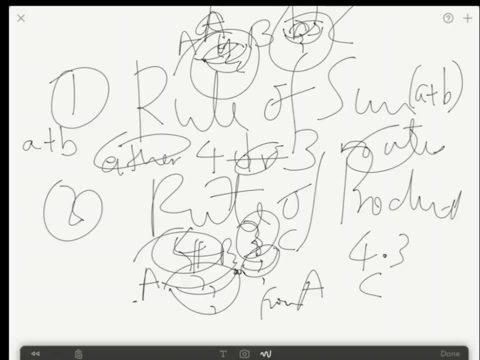 So we can say: when there are A ways of doing something and followed by that there are B ways of doing the other thing, So for each of the A ways there are B ways of doing the other thing, Then the total number of ways of doing that thing is A times B. 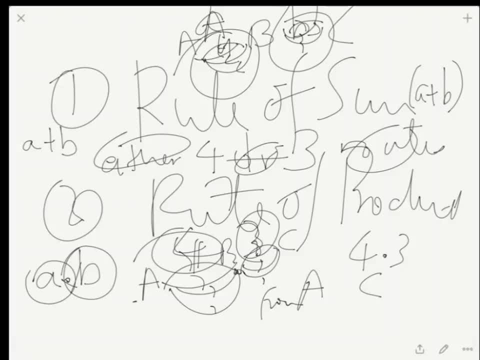 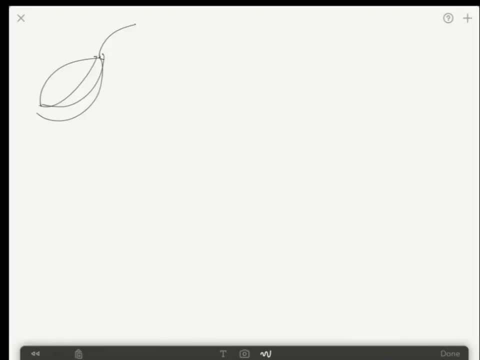 So let me give you one more example over here. Let me organize this One for all. So if there are these four ways and three ways, then four ways and three ways. If you want to get out of B, there are four ways plus three ways. 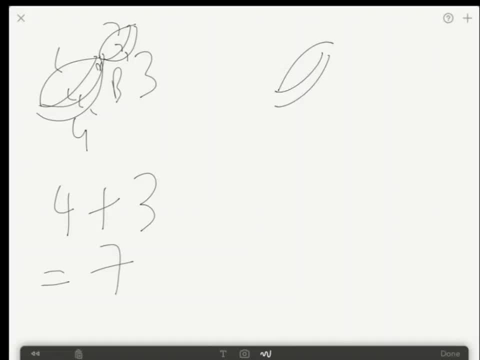 That is, there are seven ways. If you want to go from A to C, then there are four ways of going from A to B, And then for each of the ways, there are three other ways to go from B to C. 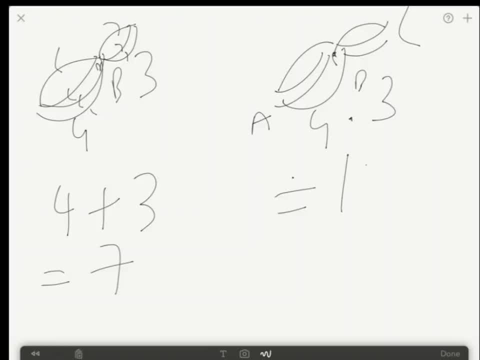 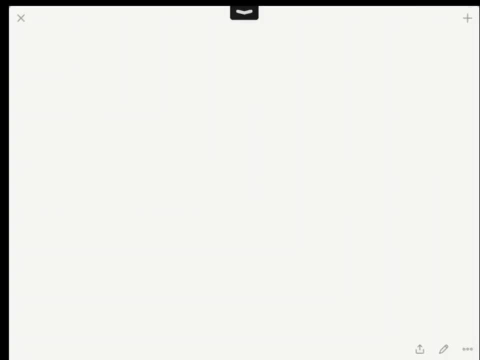 So there are all in all Four in four, 4 into 3, there are 12 ways of going from A to C. Similarly, we take another question, just quite similar, but this will help you distinguish between these two rules. 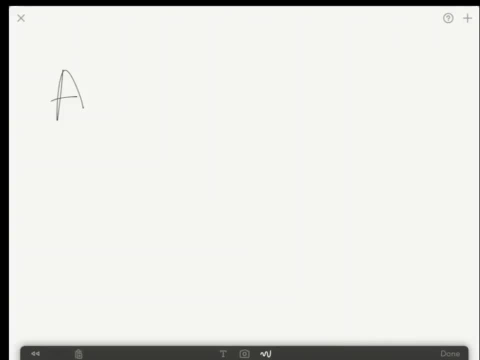 If there are A ways of going. if there are, okay. this is the other question: If there are 5 shirts and 5 full-sleeve shirts. so there are 5 full-sleeve shirts and full-sleeve. 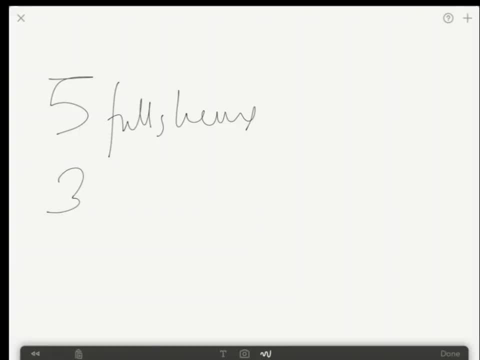 and you've got 3 half-sleeve shirts, then what are the total number of shirts that you can wear? It's simply: I have 5 ways of wearing a shirt and 3 other ways of wearing a shirt, or you have 5 ways of wearing a shirt or so. or is an important thing? either, or 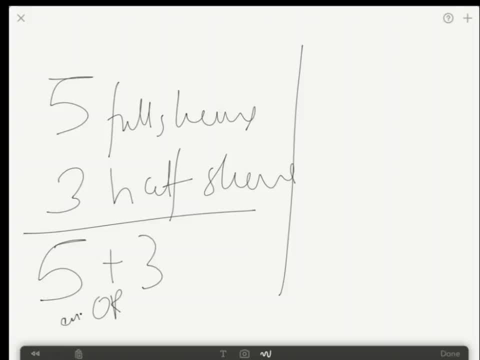 So either you have 5 ways of wearing a shirt or you have 3 ways of wearing this other kind of shirt. The total number of ways of wearing a shirt is 5 plus 3, which is 8.. Now you have 5 shirts and 3 trousers.